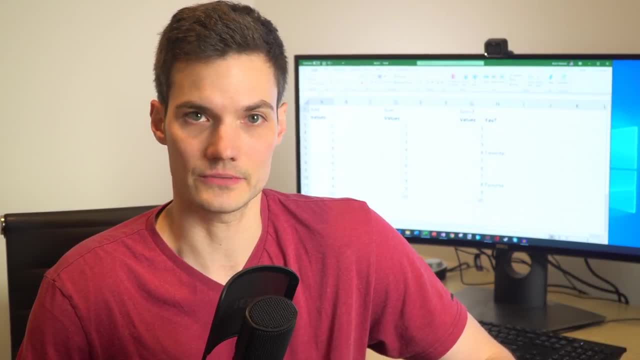 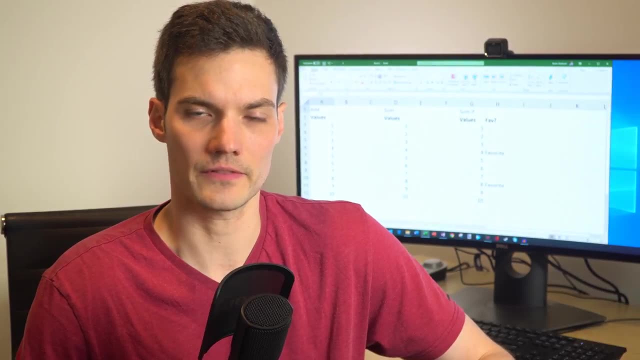 co-worker call me into his office and I said: all right, let me go in there and see what's going on. and he said: oh, Kevin, you know I'm working on this spreadsheet here and it always just takes me a long time to add up these different values. I kind of looked at him and I was like: okay, you know why. 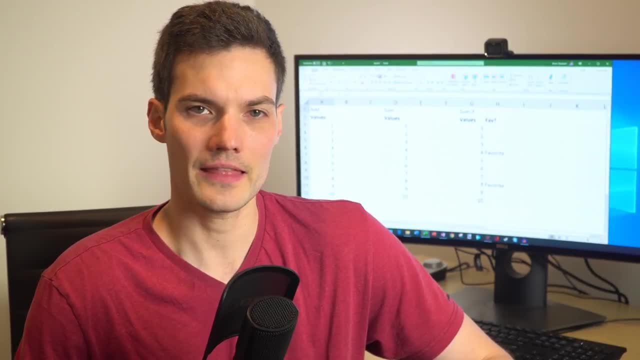 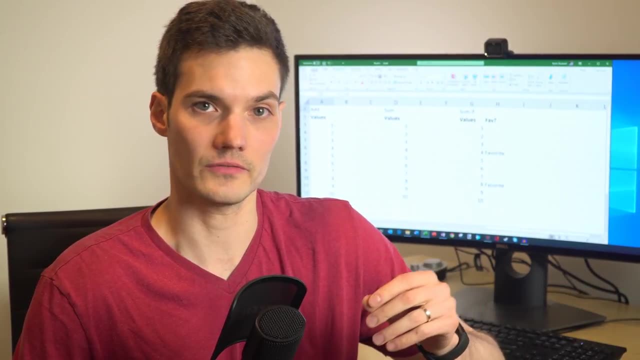 does it take so long You're using a spreadsheet makes it pretty simple for you. And then that's when I noticed that he had a calculator sitting alongside his keyboard and he would go through the spreadsheet cell by cell and when he saw the value he'd type it in. and he'd type it in, and 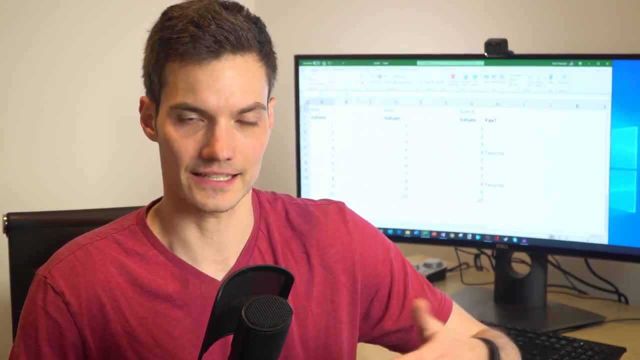 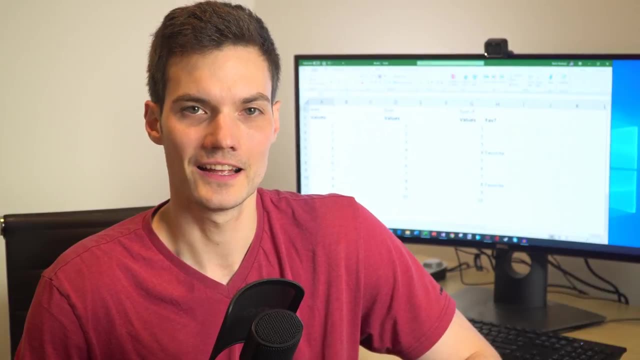 put it into his calculator. Then he'd add the next value, hit the plus button, take the next value, add it up, and then he would get the SUM on his calculator and then he'd paste it. Once he got the SUM, he would paste it back into the spreadsheet. Now, that is exactly what a spreadsheet is supposed. 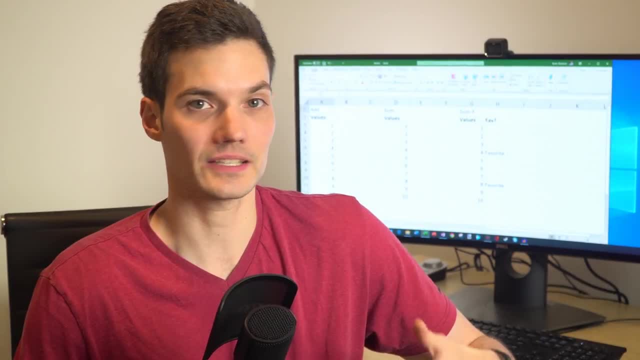 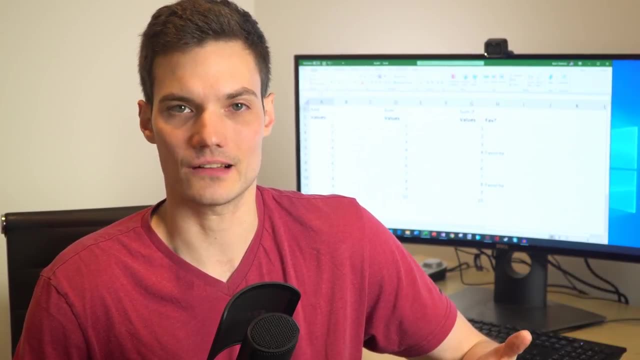 to do for you, and so today I want to basically pass on how you do this in Excel. So enough talk. why don't we jump into Microsoft Excel and I'll show you exactly how to sum up values Here. I am on my PC, I'm in Microsoft Excel. 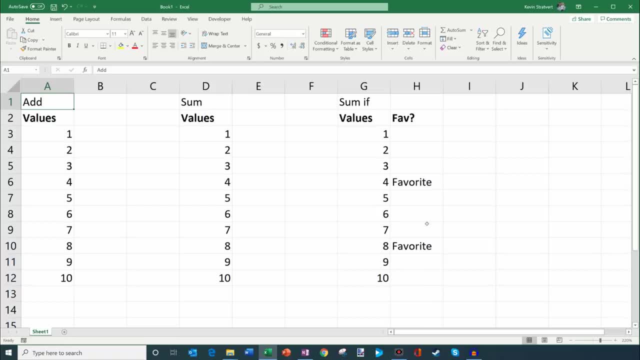 This is the latest version that comes with Office 365, but even if you have an older version of Excel, you should also be able to do this. I have three different columns. we're going to jump through one by one and how you basically add SUM and then SUMIF, and I'll get into what. 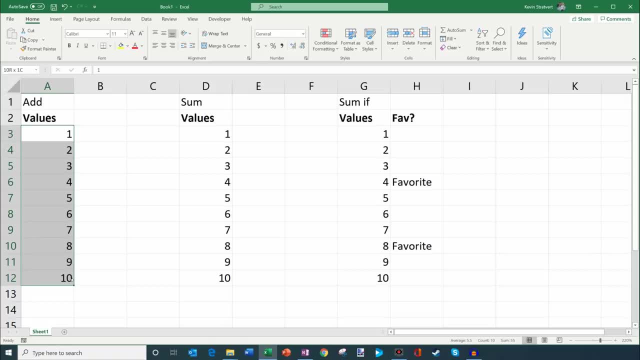 those mean. So in the first column I have these. I have basically the numbers one through ten, and we want to add them up. Well, how do you do that? Well, that's in Excel. you could enter what's called a function. I'm going to enter the equal sign. you always start. 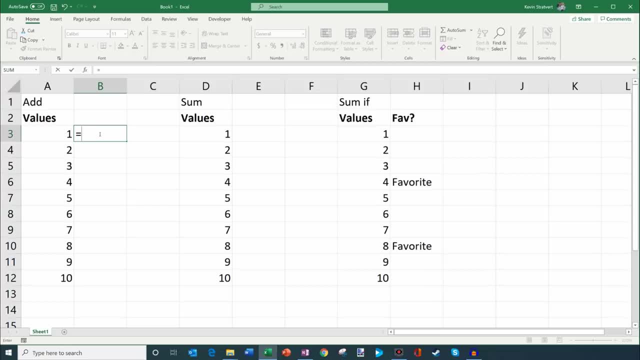 a function with the equal sign. So first we're going to do equals and what I want to do is, let's say, I just want to add the first cell with the second cell. Well, what I do is I click on the first cell, which is A3, and then I'll insert the plus sign and I'll do cell A4, and then I can hit enter and 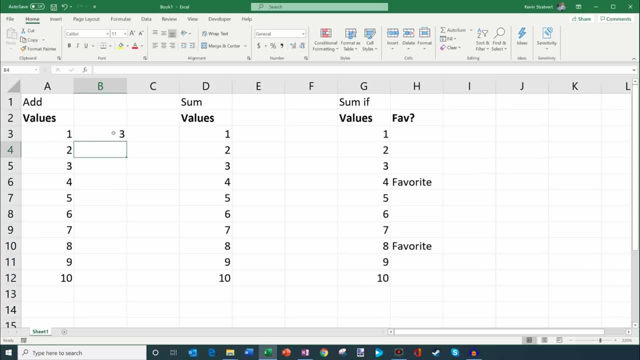 that'll add the two values. So one plus two is three- at least hopefully most of you agree with that- and that gives me three. And what I could do is, let's say, I wanted to add this whole list. I could go through and I could say: well, this cell plus this cell plus this. 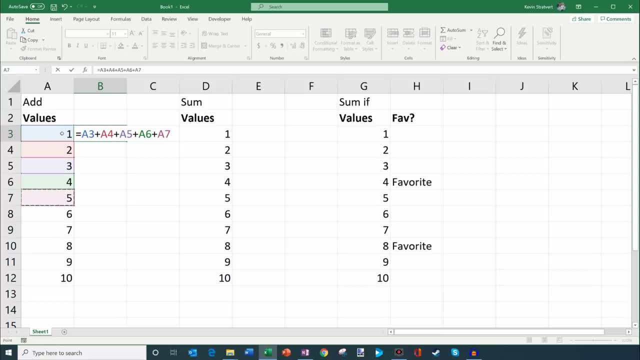 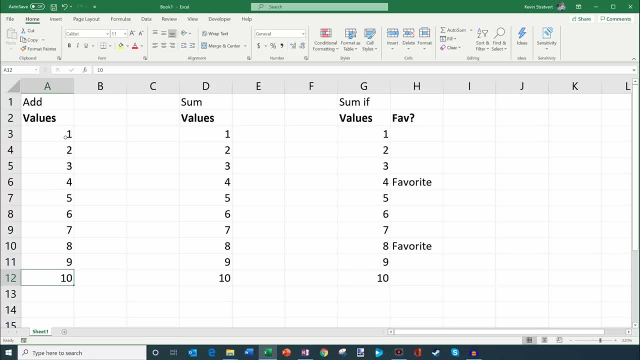 press enter, And so adding is very good when you only have a few values that you want to add, but as soon as you have a lot of values, it doesn't scale all that well, And that's where the sum function comes in. So what is a sum function? Well, why don't we first click? 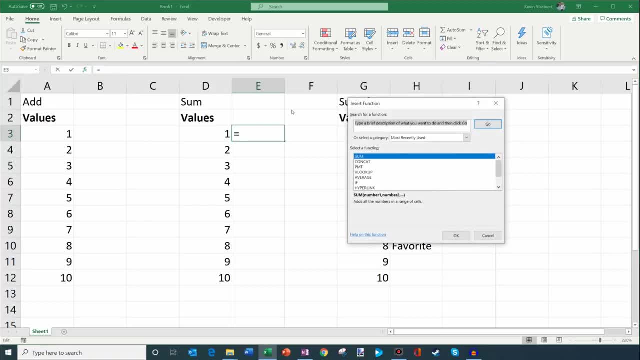 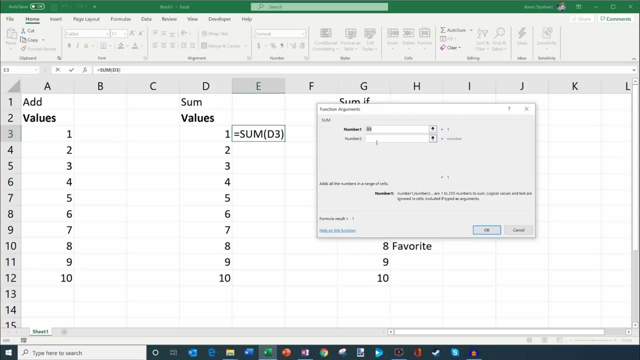 on the function icon up here where I can insert a function, and I'm going to search for sum. You'll also see that it's a recent function that I use, So I'll just go ahead and click on that, And what you could see here is it. 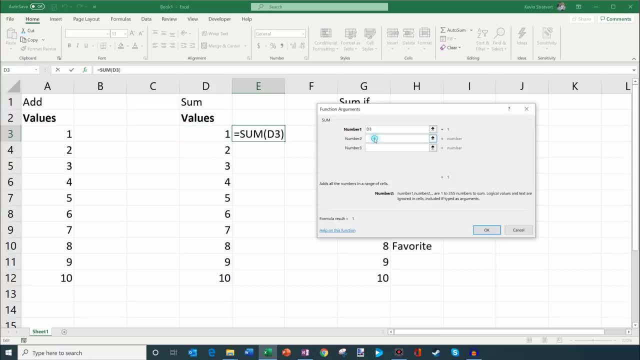 says: well, you know, tell us number one that you want to sum. Well, I want that one. And then for number two, I want to sum that cell. Number three, I want to sum this cell. And I could go through all my numbers and just keep doing that all the way down my list. and 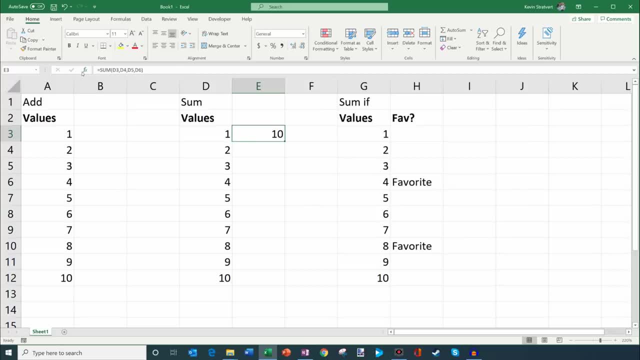 then click OK. The problem, though, is that, too, if I click through using the insert function tool, that also takes a little bit of time. Now, what you could see is, when it created that function, it does the cell followed by a comma, followed by the next cell. So what? 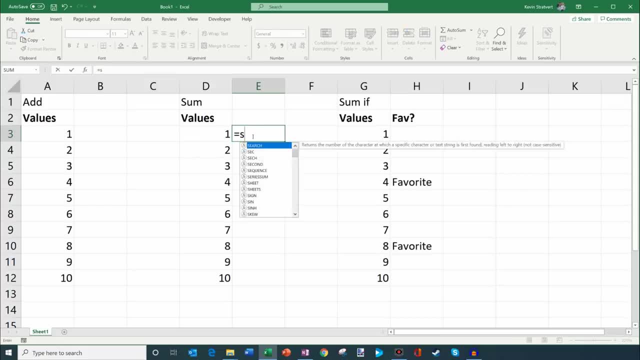 I could do as well is: let's type in the formula, So I'll do equals and then sum, open parentheses, And then I could click on this cell followed by a comma, And then I can go through and click on all the numbers that I want to sum. This is probably just as much. 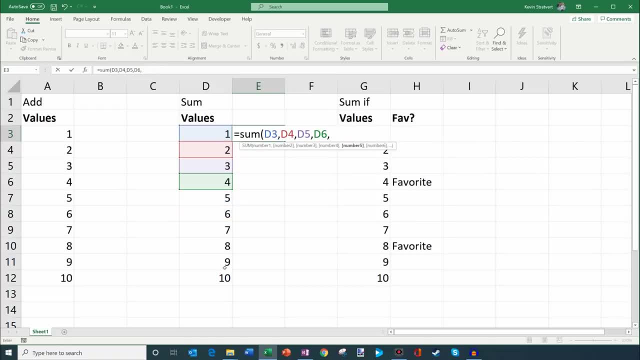 effort as entering a plus sign, though. So how do I make it even easier? What if I just want to sum this whole list? Well, what you could do is I'll type in the sum function. So equals sum, open parentheses. 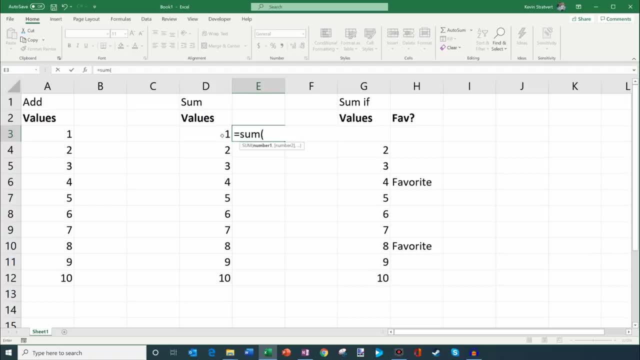 And what I can do is, instead of entering one by one, what I could do is I'll click here and I'll just drag it all the way down, So you see that I put a colon in between, And what this is saying is that I want to sum everything between cell D3 all the way down. 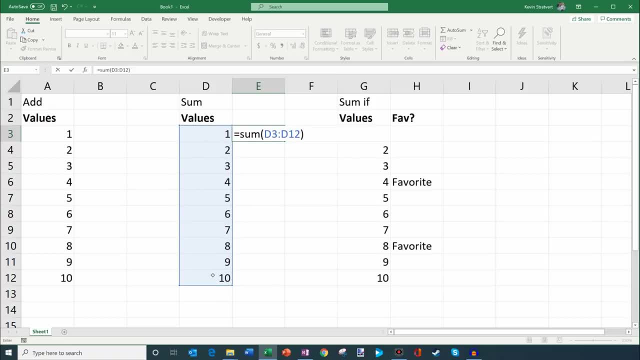 to cell D12. And then I'll close the parentheses and hit enter. And what that did now is that summed up every single value in here. So pretty cool. Now what I can also do is I'll type in equals sum again, And what I'm going to do is, let's say, I want the first three values. 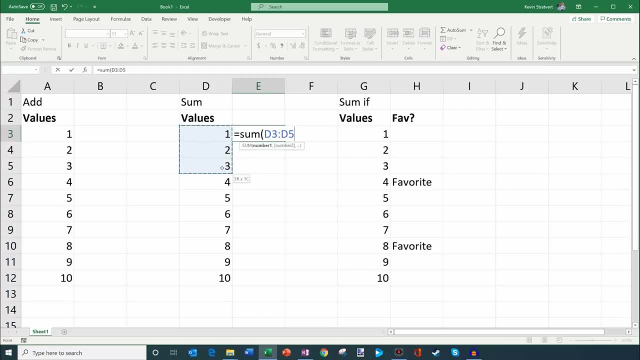 and I want to sum the last three values. So I selected this range, so D3 through D5.. And now what I can do is I'll enter a comma And now I can highlight the next three down here, And then I'll close the parentheses. And so what that did now is it sums these. 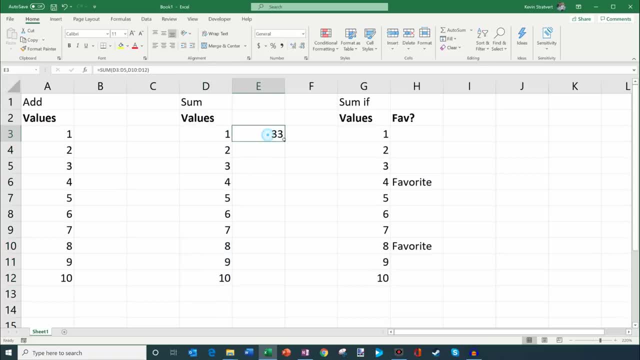 three values and then it also sums these three values. And what's really neat is, with the sum function I can highlight a few values here put in a comma, highlight some here put in a comma, highlight some here, highlight some here and highlight some here and then 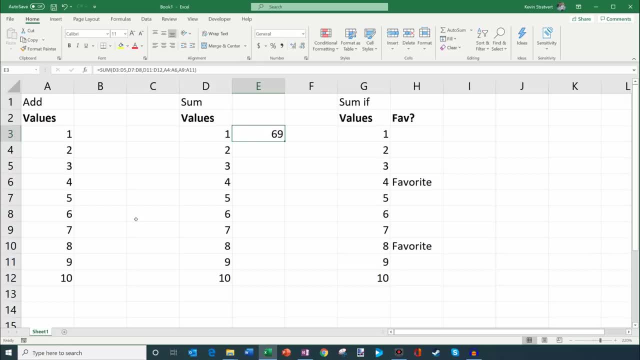 close the parentheses, So I can add a lot of things very easily by using the sum function. So pretty, pretty cool stuff in terms of addition. Now what I also want to show, though, is what, if you only want to sum up certain values- Like, let's say that I only want to sum my favorite numbers- 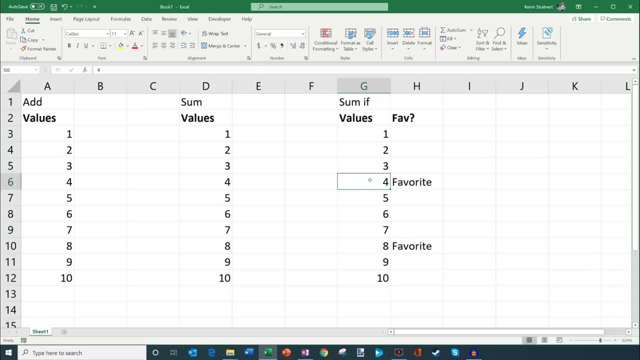 between 1 and 10. And that happens to be 4 and 8. Actually I just made that up, But let's say those are my favorite numbers: 4 and 8.. And I want to just sum those values. 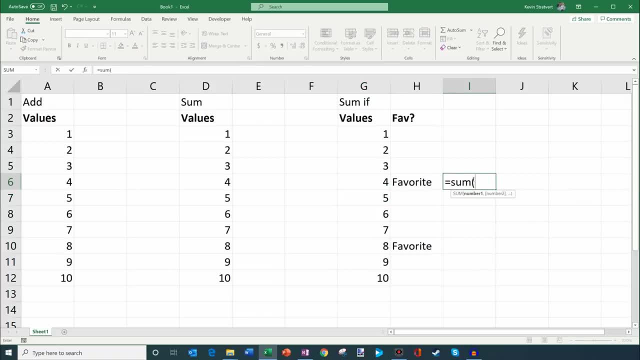 Well, what I could do is, you know, once again I could type in equals sum And I could say: well, 4 is my favorite value, And then comma 8 is my favorite value, But once again this doesn't scale very well. 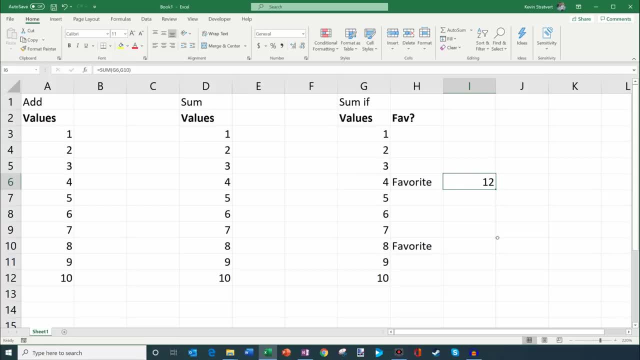 Imagine that you had thousands and thousands of rows of data. Some are favorites and some aren't favorites. Well, what comes in? what you can use here is sum. if. So, what I'm going to do is: why don't we go to the insert function up here and I'm going to type in sum if? 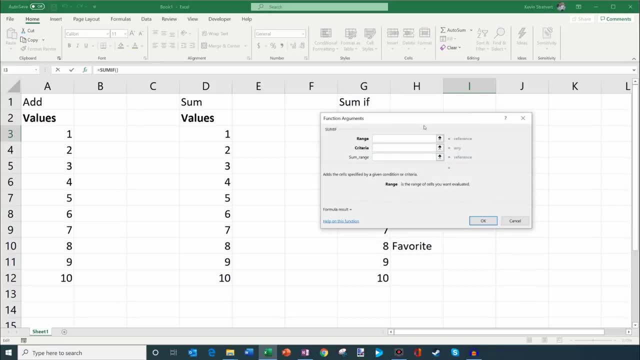 And then I'm going to click on go and that brings up this sum. if function, Let's go ahead and click on OK. Now I'm confronted with a few different options here. One of them is the range. Well, what does range mean? 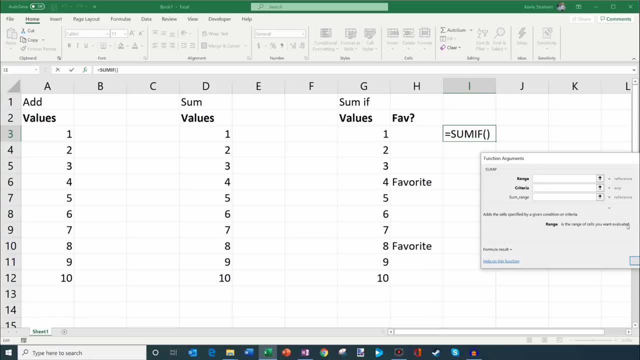 Well, here it says: the range is the range of cells you want evaluated. Well, what I want to do is: I want to evaluate. if this is my favorite, So for the range. why don't we select this favorite column? This is my range that I'm evaluating against. 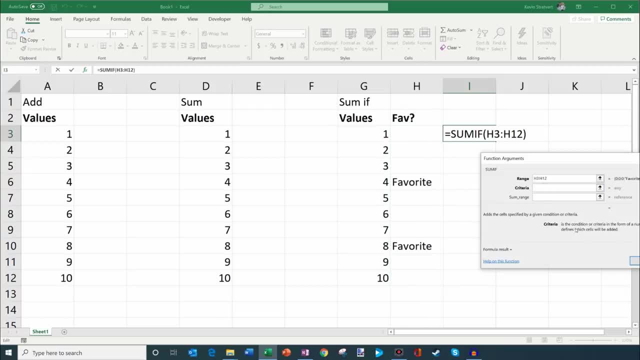 The next option here says the criteria, And this is the condition or criteria in the form of a number expression or a text that defines which cells will be added. Basically, what that means is: what am I looking for in these cells? And what I want to do is I want to.